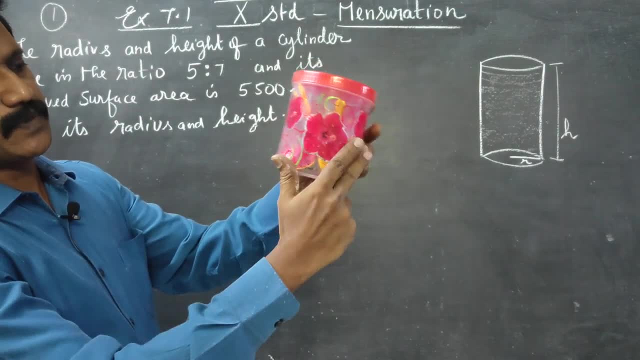 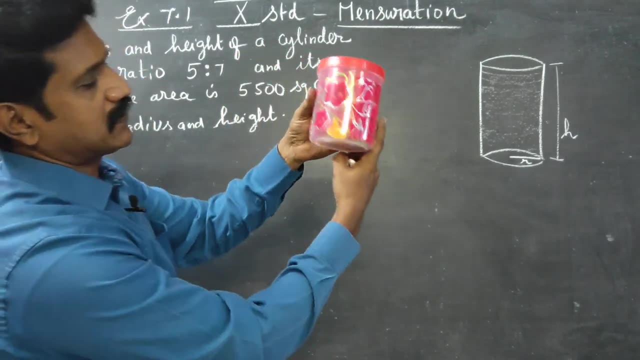 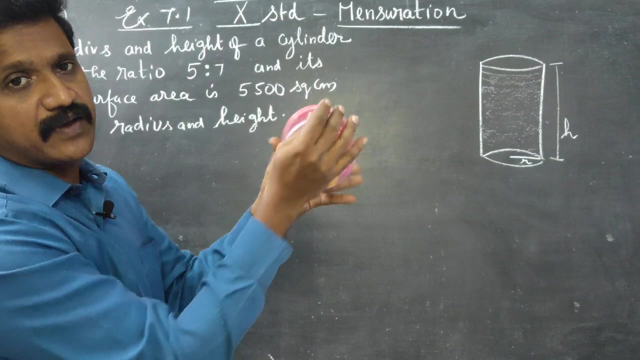 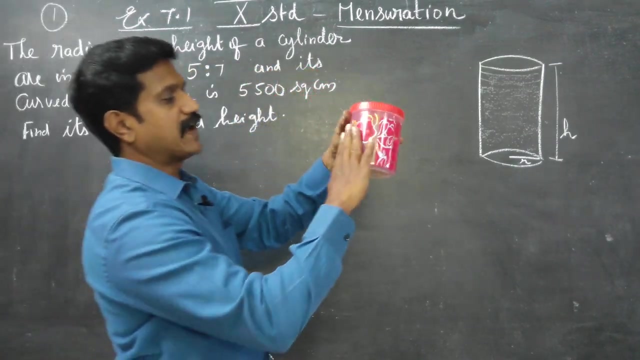 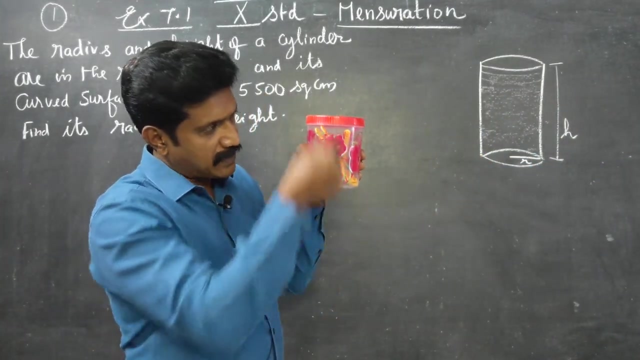 See here, see here. Now let's see Bend-Bend surface area in the rotation path in the volunteer to the partner Karuna, in the top or on the bottom water. it could burn the height, the measure: funny party night radius in getting a center point. 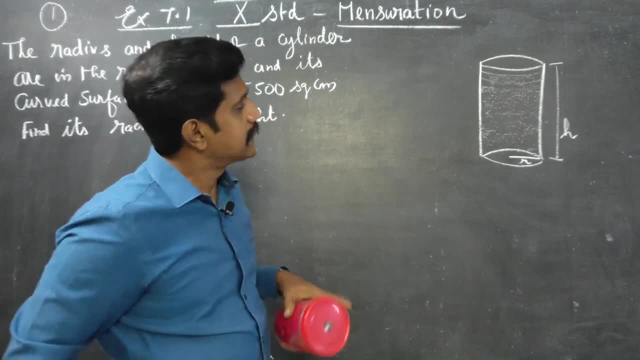 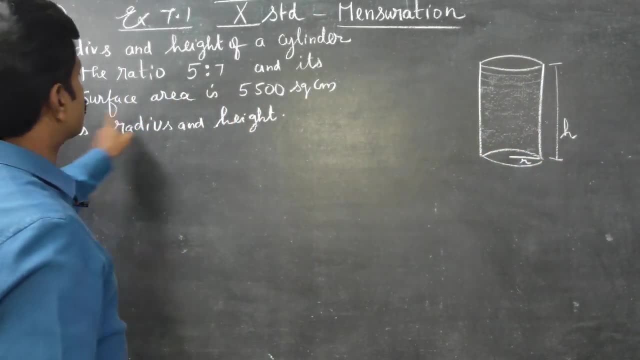 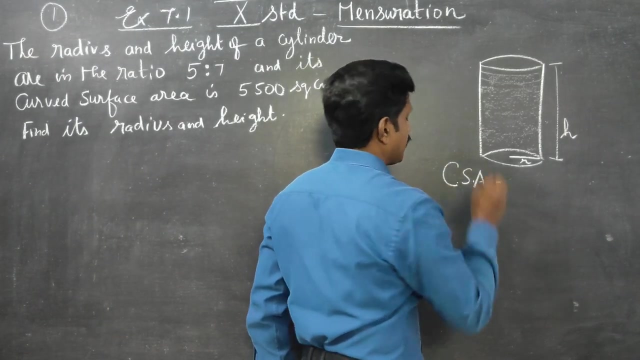 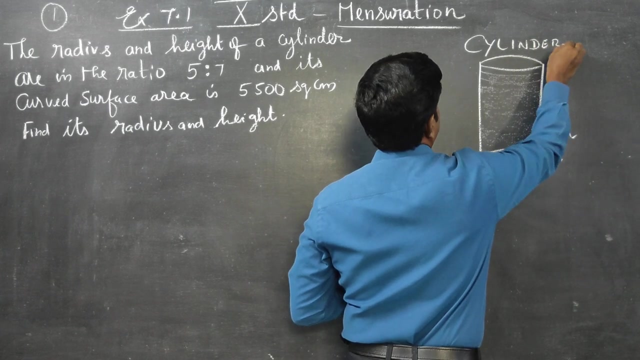 learn to the corner. very good radius high school to come and I'm a kind of radius put together hi to radius of ratios. look at the current surface area. the answer to that today you are going to know. the first formula: see, yes, he means curved surface area of cylinder. curved surface area of cylinder 2 pi R. 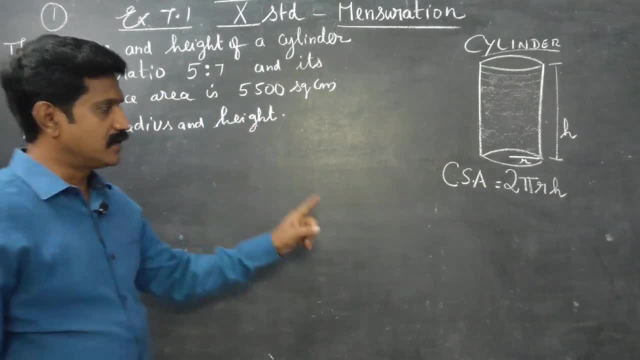 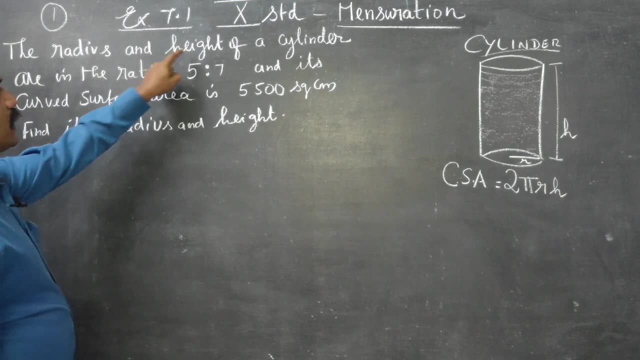 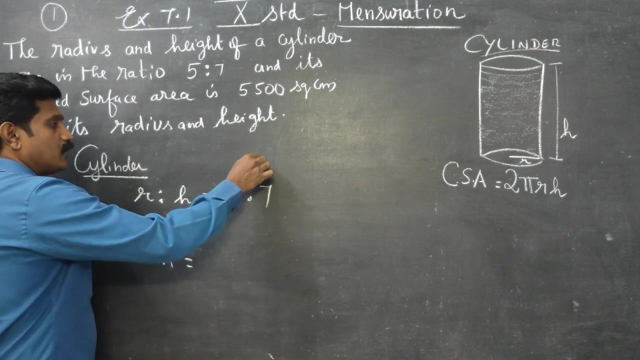 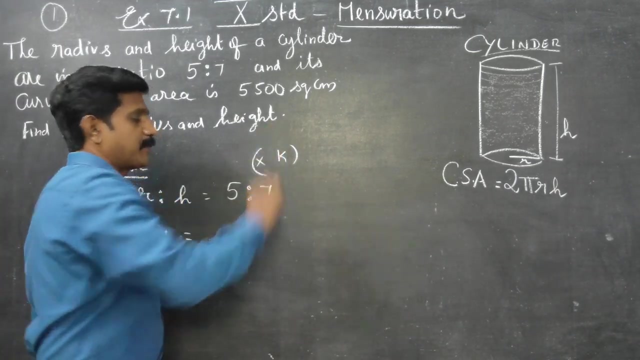 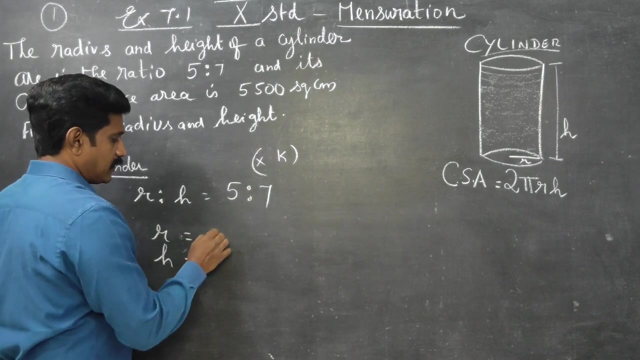 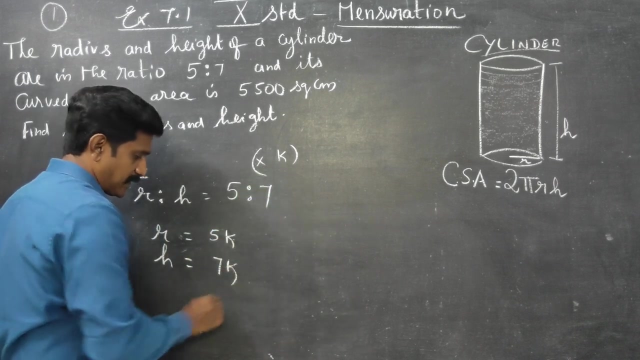 H 2 pi R. H is the curved surface area of the cylinder. with this formula- I'm going to enter into the some radius of height or ratio to come- my C- the ratio break up I don't about- is equal to 5k. H is equal to 7k. CSA curved. 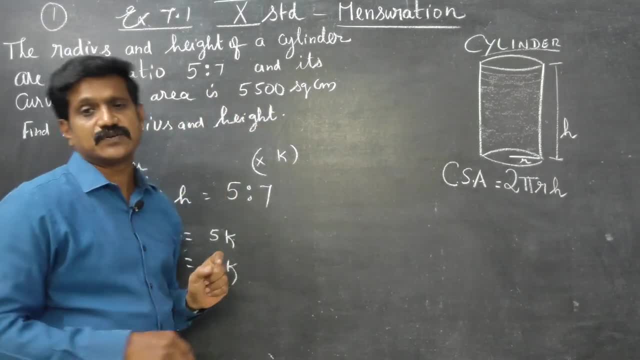 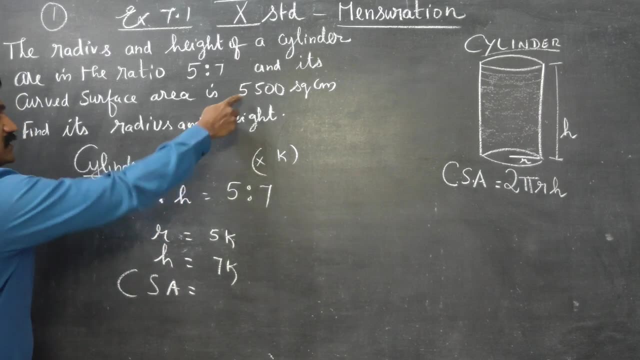 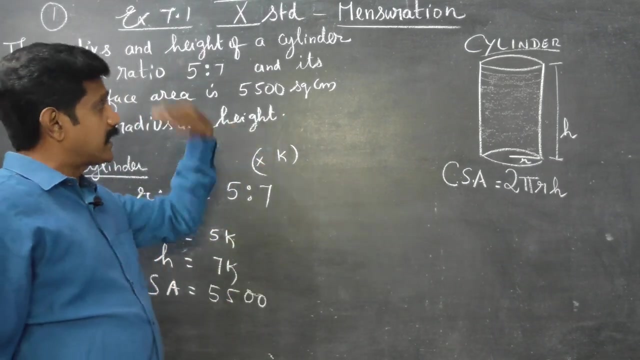 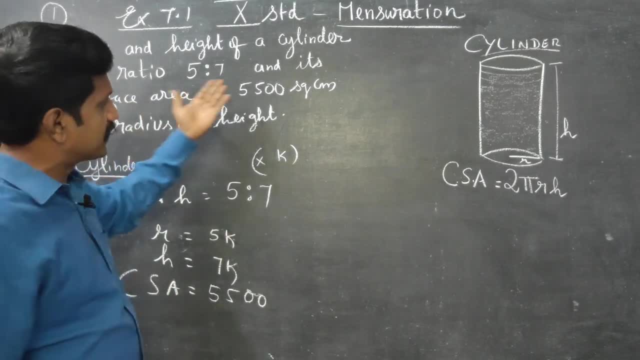 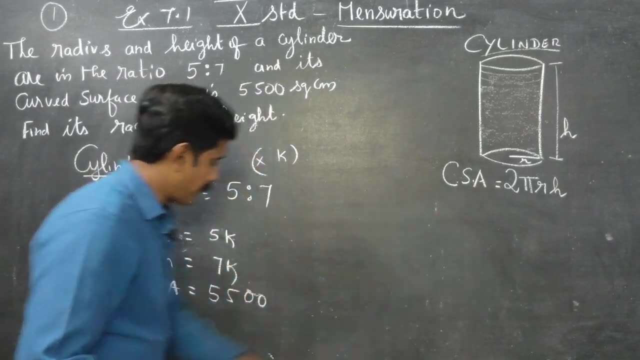 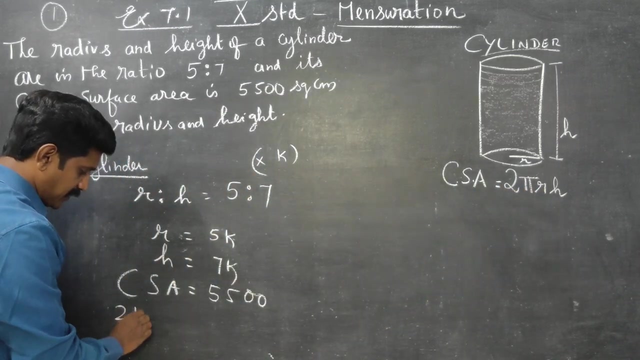 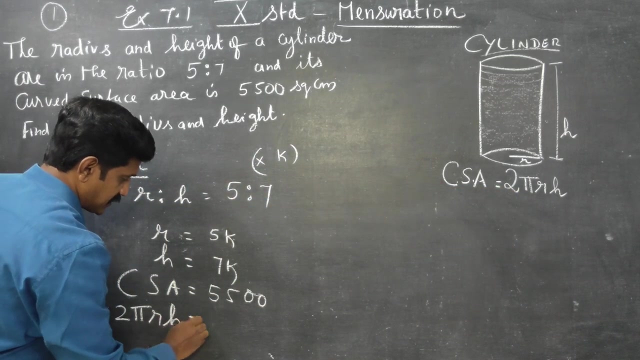 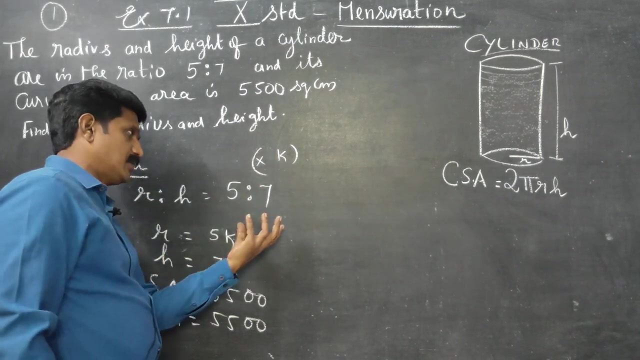 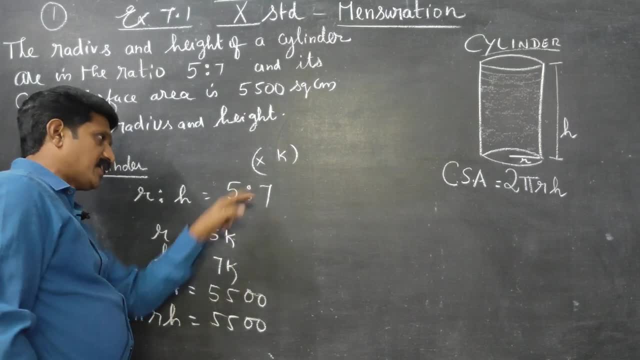 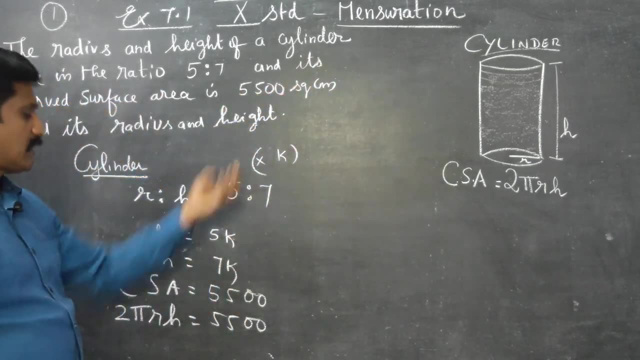 If you multiply by the same letter, then 5 into k is 5k and 7 into k is 7k. The ratio is broken. The answer of CSA is given as the value 5, 5, 0, 0.. 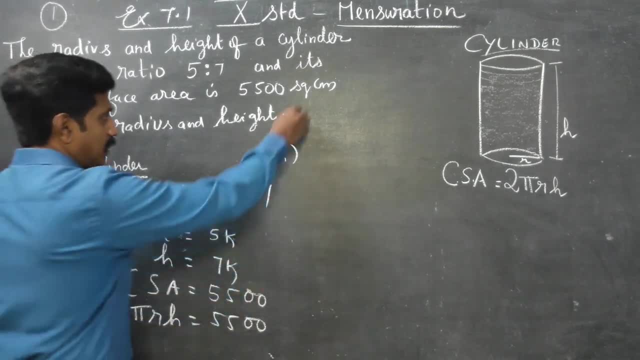 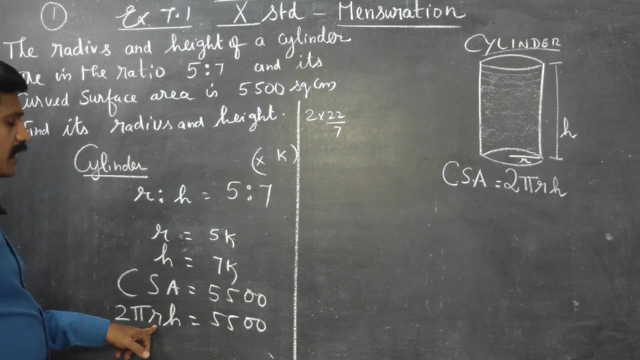 So I will write the formula of CSA there: 2 pi, r, h. I will write the formula 2 into: pi means 22 by 7 h. in that sum the value of r is 5k. 5k into h's value is 7k is equal to 5, 5, 0, 0. 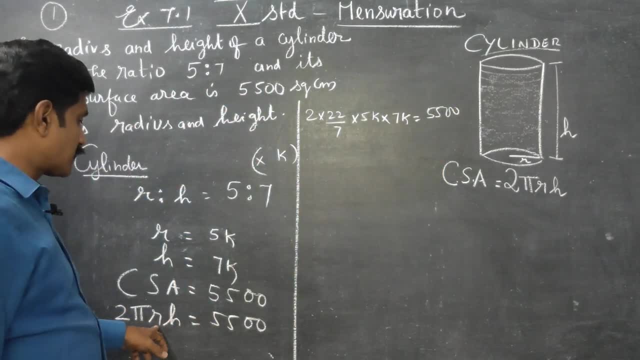 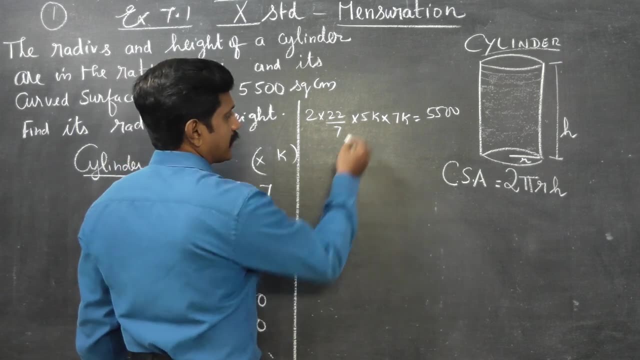 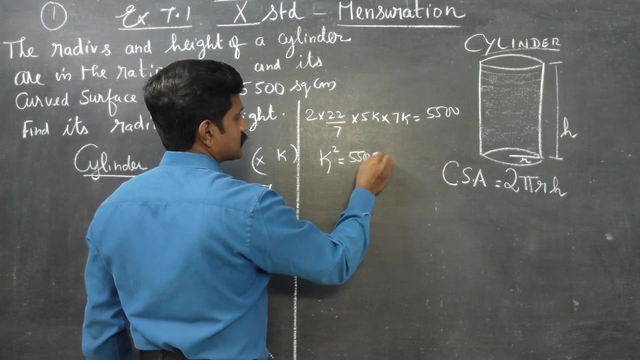 What did you do, sir? Instead of pi, you have written 22 by 7.. Instead of r, instead of h. r is 5k, h is 7k. I have substituted: When you start simplifying k into k, is k square is equal to 5, 5, 0, 0, into 7.. 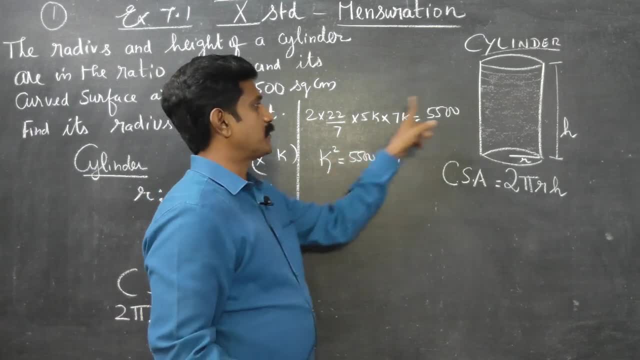 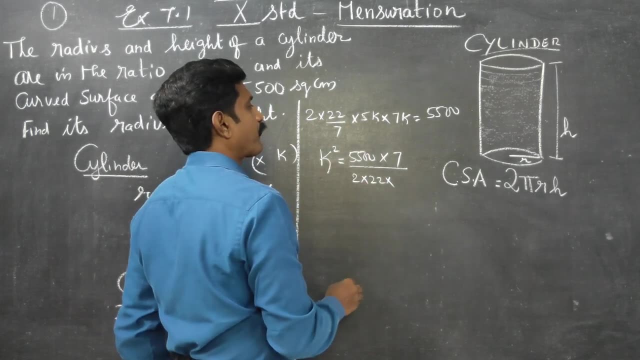 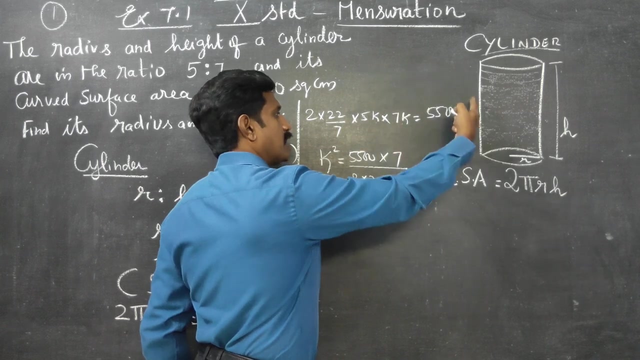 I have sent the 7 in the denominator to that side. The 7 below went up to that side, also The number above. I have brought 2 below 22 below 5 below 7.. Everything in the numerator will go to the denominator. everything in the denominator will go to the numerator if you change that side. 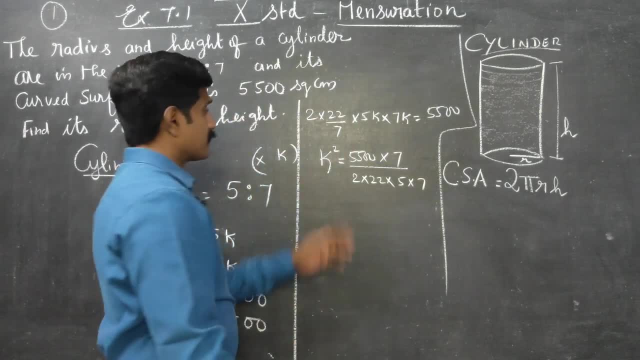 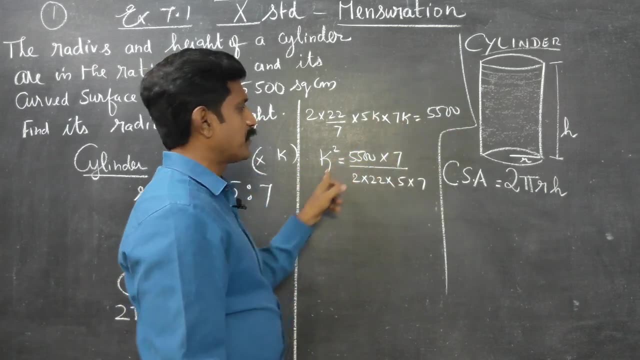 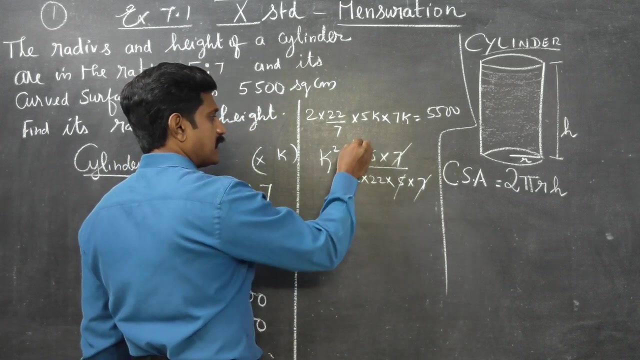 If you change that side, then when you change the numbers, all the numerators goes to the denominator. everything will be in the numerator. What did k into k become? k square 7tables, 7 times canceled 5tables. this is 1 times 1 times 0, 0.. 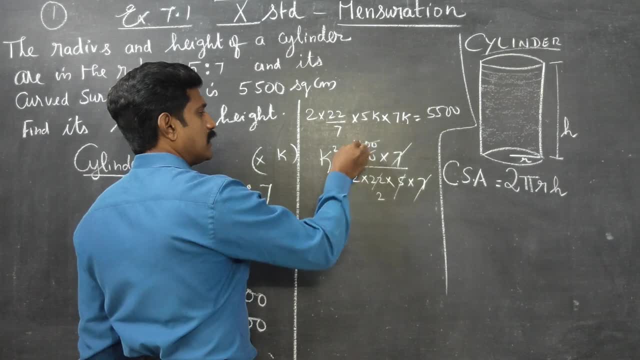 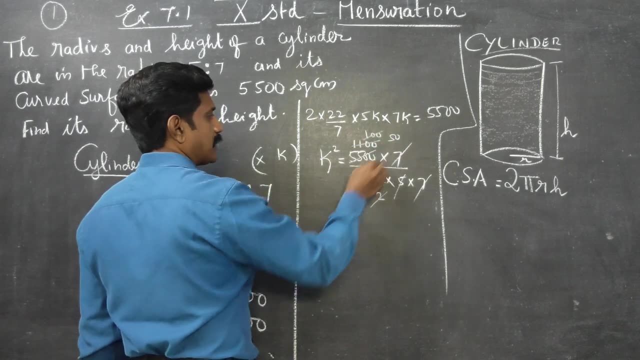 Levern tables. Levern tables is published 2 times. 11tables is published 100 times. if you multiply 1 times, 2 is 0,. 2tables is published 50 times. two tables are published 25 times. 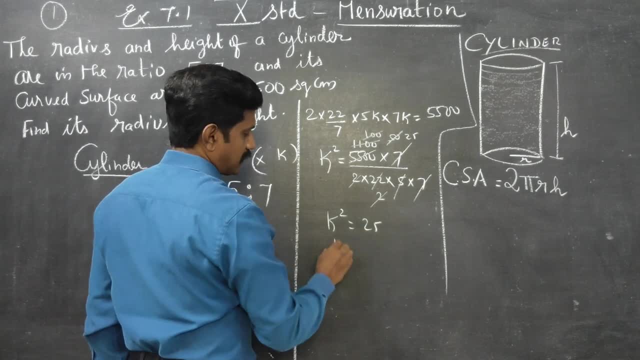 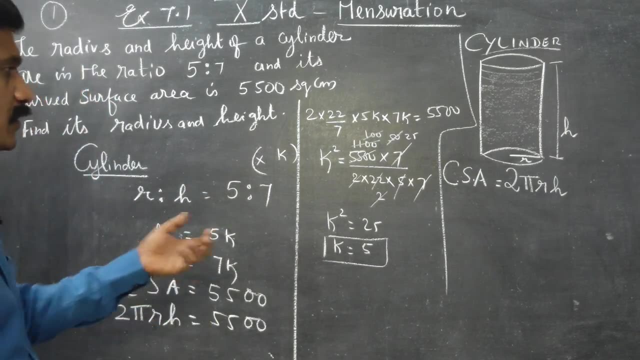 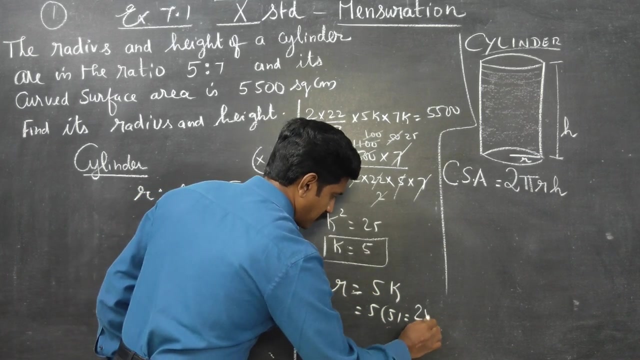 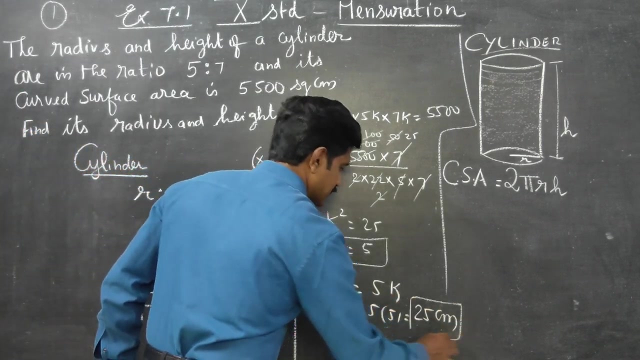 k square is equal to 25, so k will be plus or minus 5, but since this is a menstruation measurement, we will just take the positive value: k is equal to 5.. So what we will do next is to find the radius and height of k. 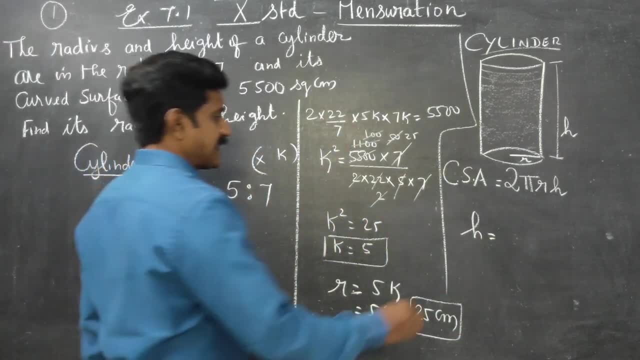 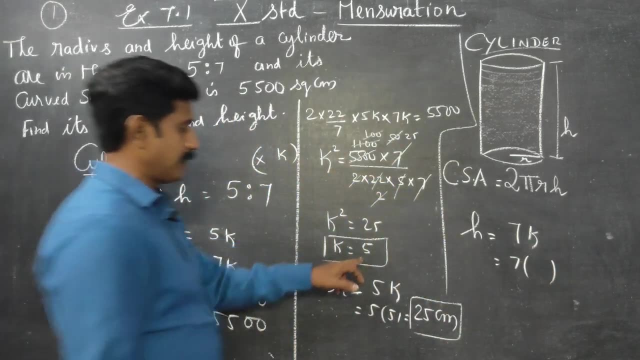 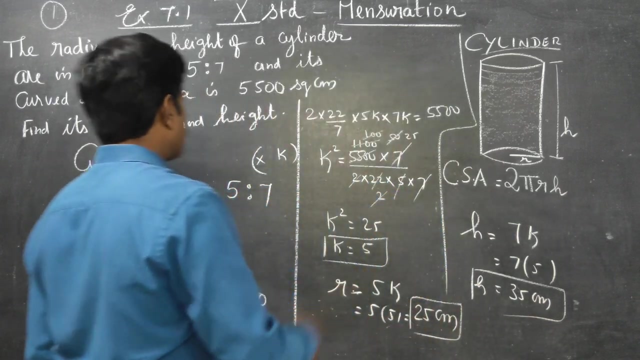 We found the radius. now we will have the height. This will be 5x5 means 25.. 7 into k, 7 into k, 7 into k's value is 5,. 7 into 5, answer is 35 cm. this is my height and this is my radius. I am going to define the radius and height. 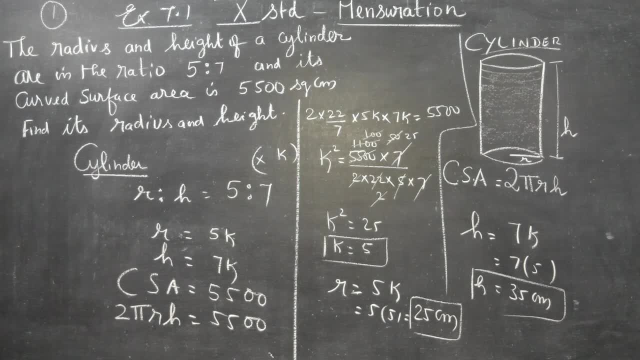 in this problem. if you know the first thing, if you break the ratio, if you multiply by any letter- k or x, if you multiply by any letter- the ratio will be broken. next, you need to know the formula CSA. formula CSA of a cylinder is 2 pi r h. CSA means the part which is straight in the cylinder. 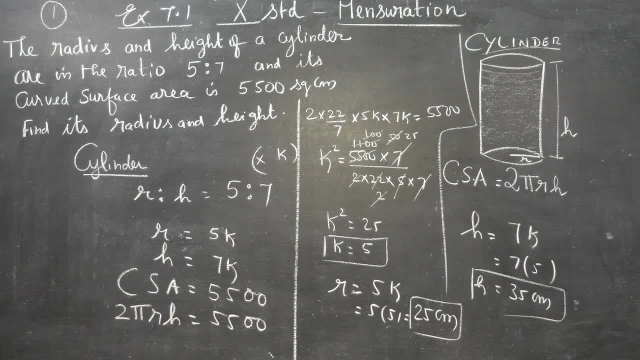 that is what we are going to find, how much paint we are going to apply or how much colouring we are going to do on it. that is CSA curve surface area. thank you.